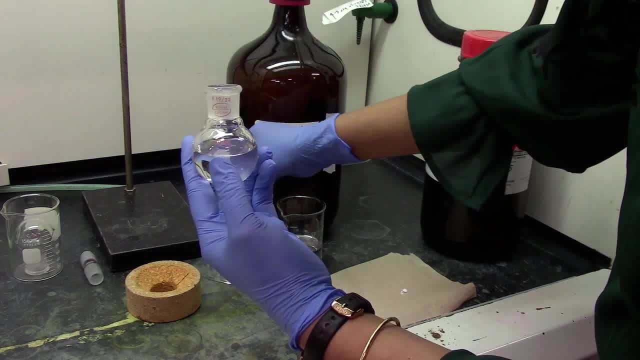 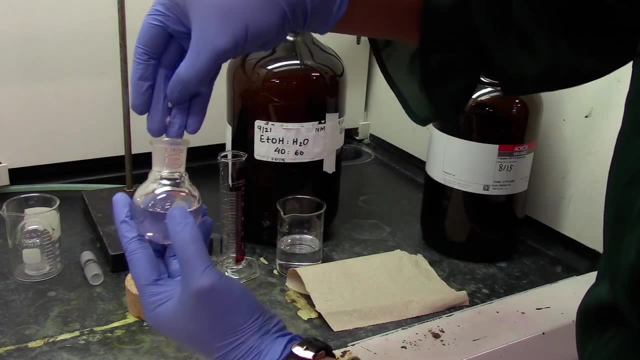 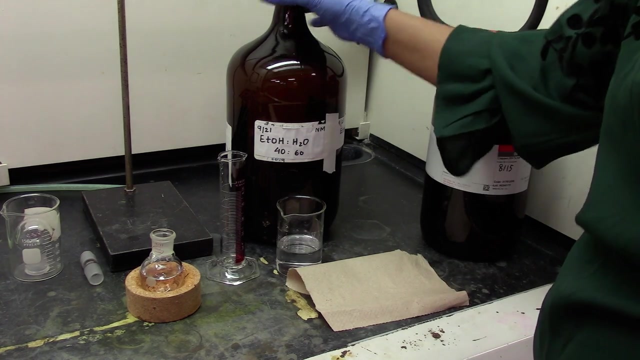 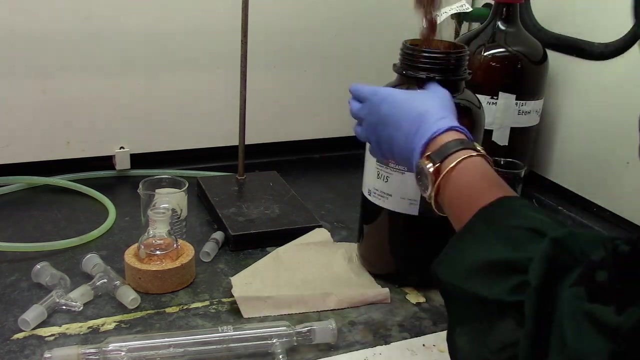 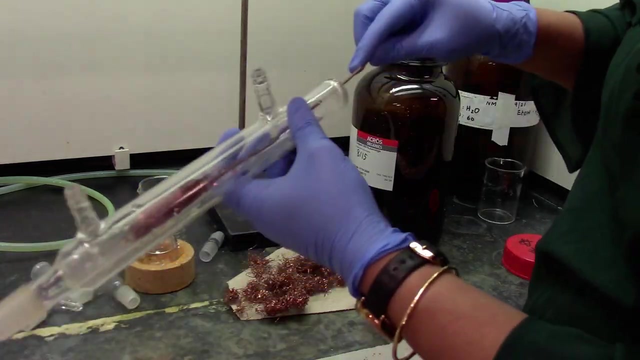 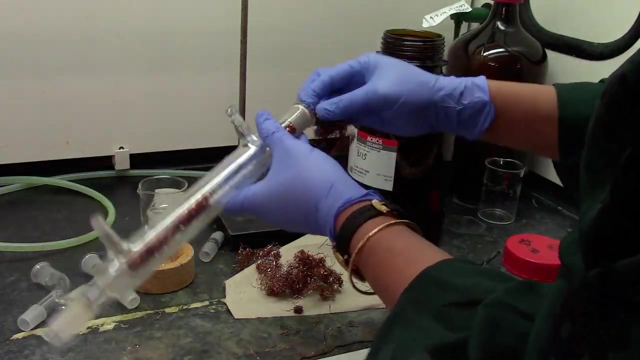 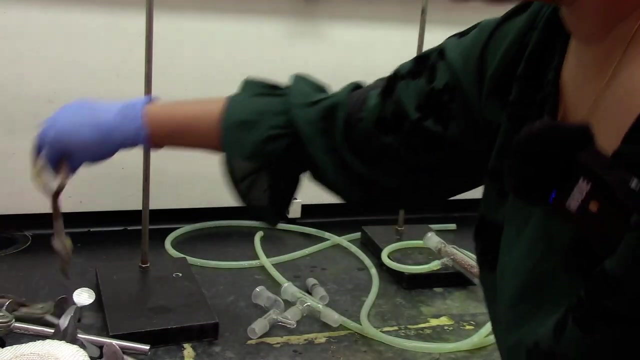 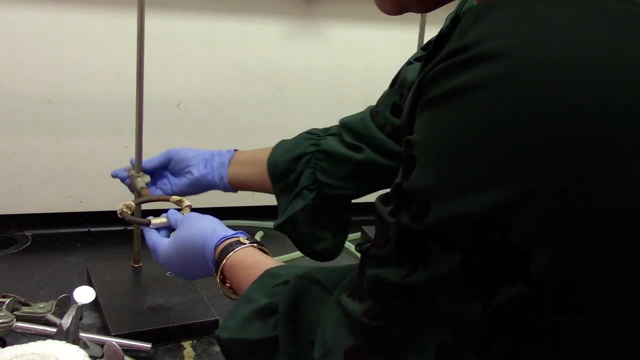 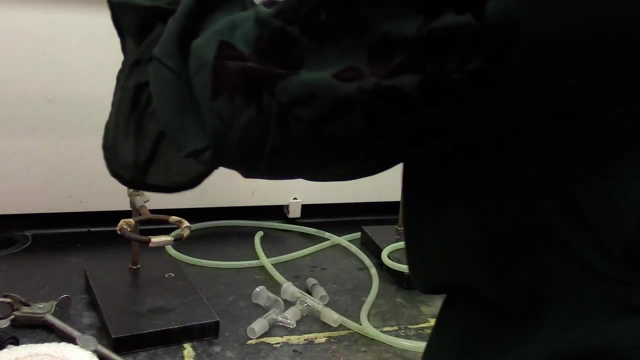 flask, which is the distillation flask. Remember to put two boiling stones. Now our starting solution is ready. Get started with packing the distillation column with some copper. We'll be packing some copper turning into the distillation column. Attach a ring clamp onto the ring stand And the clamp to hold the distillation round. 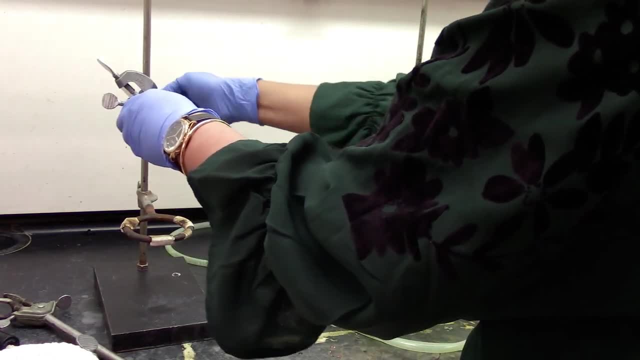 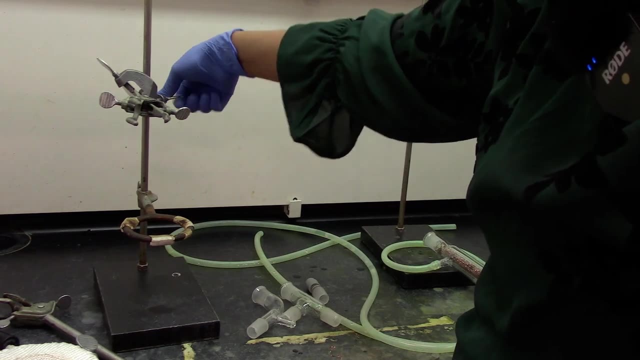 bottom flask And attach a clamp to hold the 50 ml flask. Now we're going to start by getting a 25 ml water into a 50 ml round bottom flask. Here's my mixture. Get started with packing the distillation column with some copper turning. 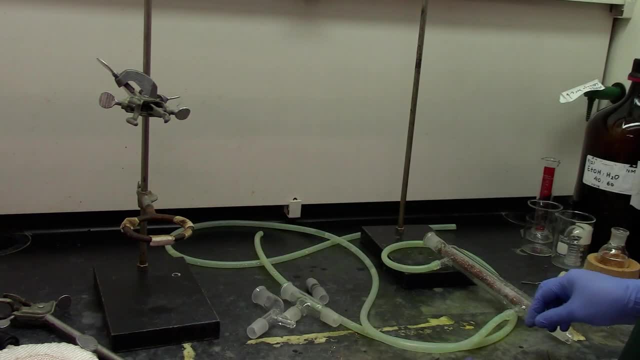 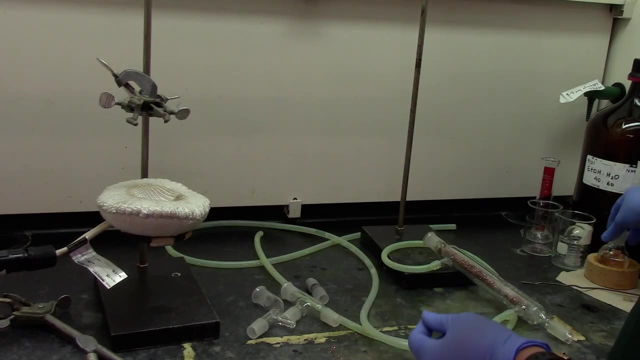 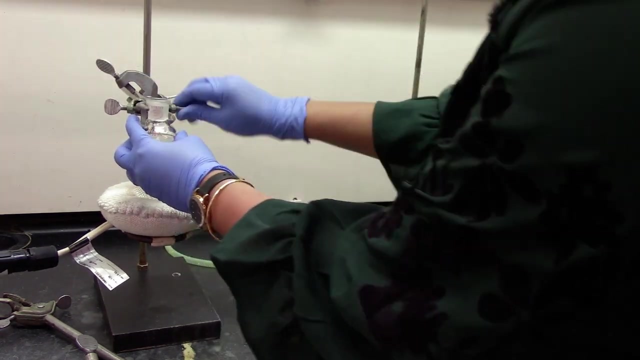 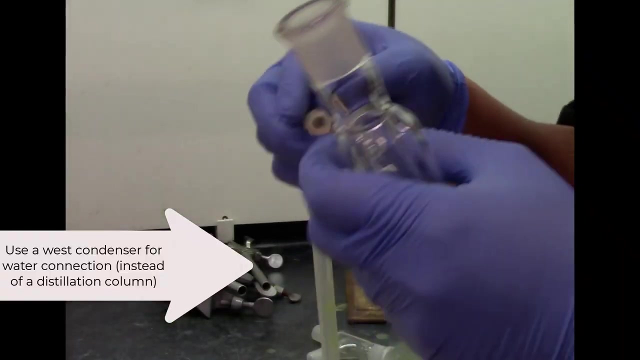 into a 50 ml round bottom flask. So this is where your mantle will be sitting And this will be attached right here Again. dip it in some tap water, which acts as a lubricant for easy attachment to the distillation column. 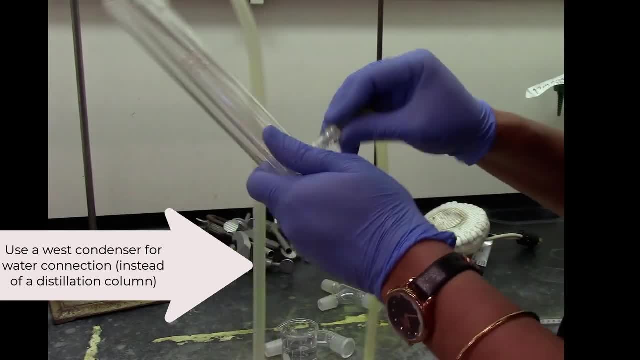 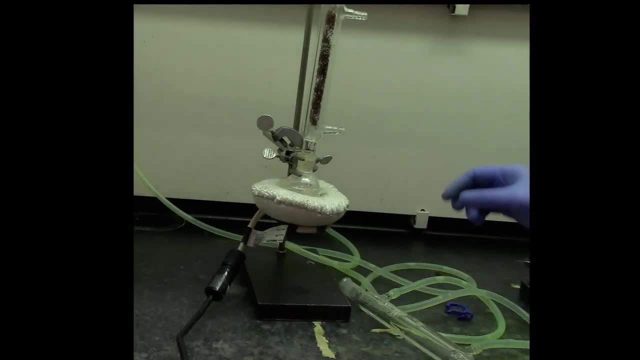 Now we're going to connect the element of the Tigon tubing into your distillation column. Once you connect your round bottom flask, place the distillation column with the copper on it And your thermometer adapter goes on top of your three-way connector and goes on. 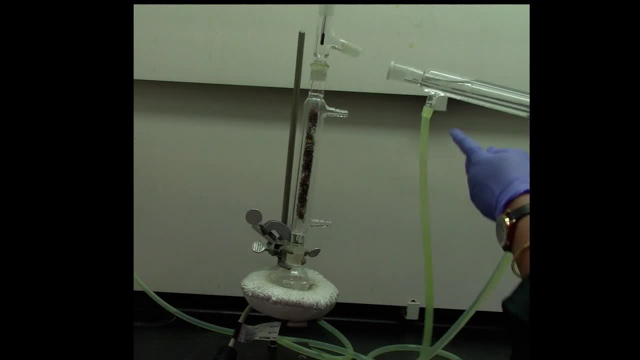 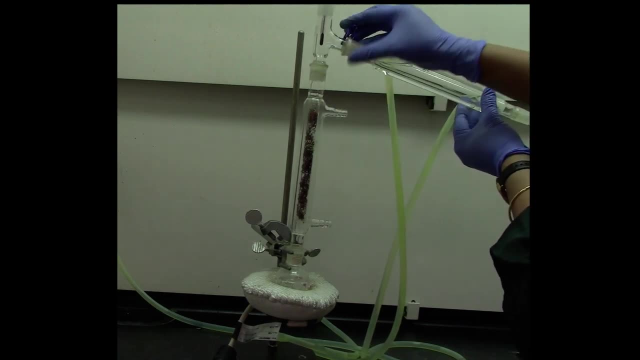 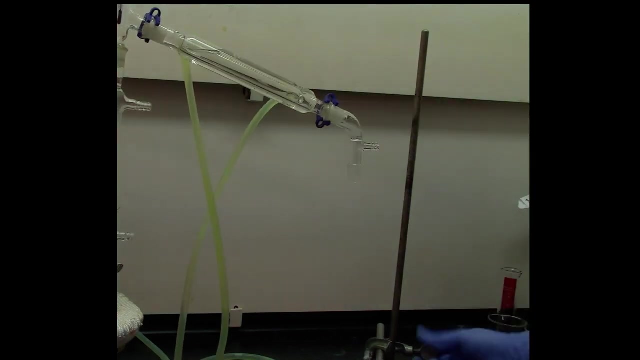 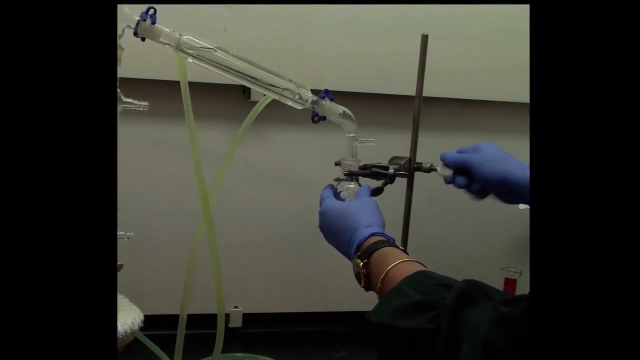 top. Now we're going to connect a condenser with the water connection. Here we have our right here. Make sure to use a keg clamp At the end, another keg clamp holding the vacuum adapter. Now we are going to put the collection flask at the end of the vacuum adapter. 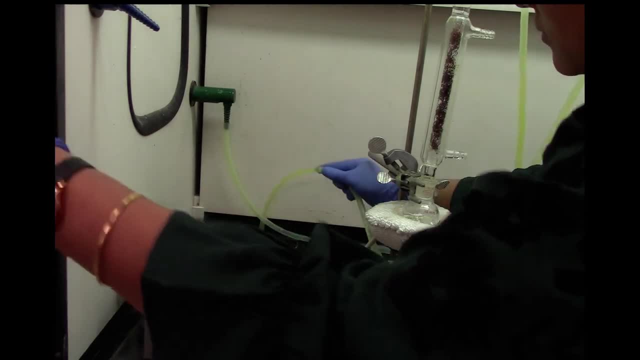 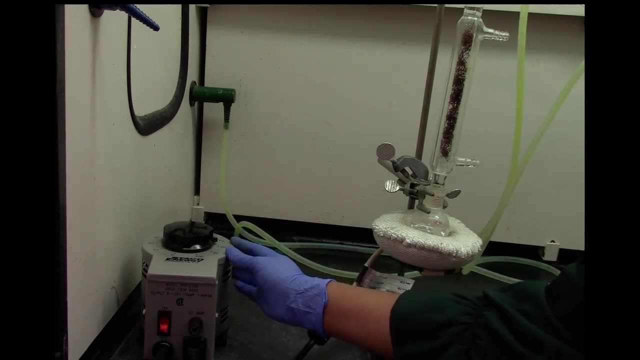 Make sure to turn on the water And now is a good time to turn on the variette. Put the variette on top of the flask And come back to the flask. put the variate between 70 to 80 percent and wait for the mixture to start boiling and distilling. 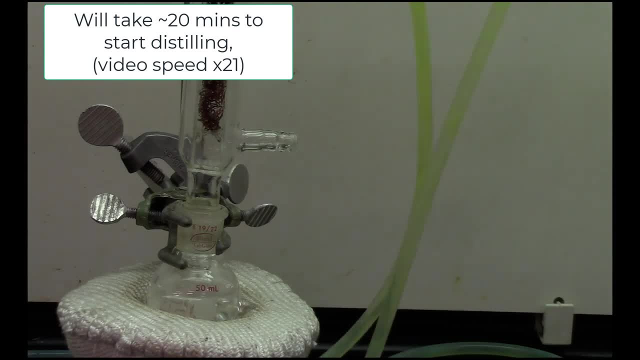 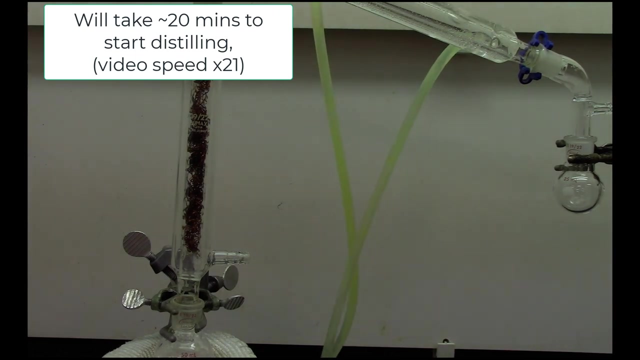 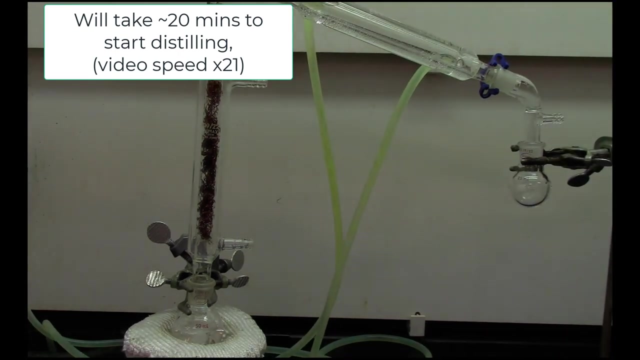 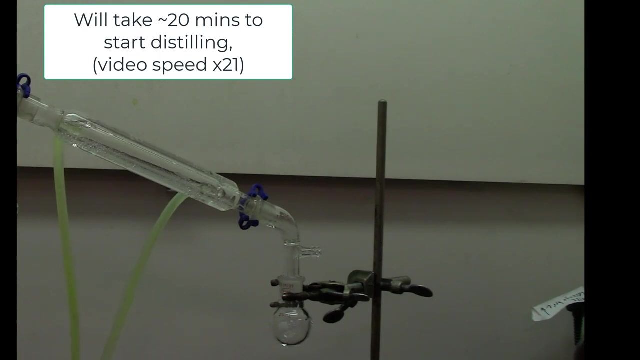 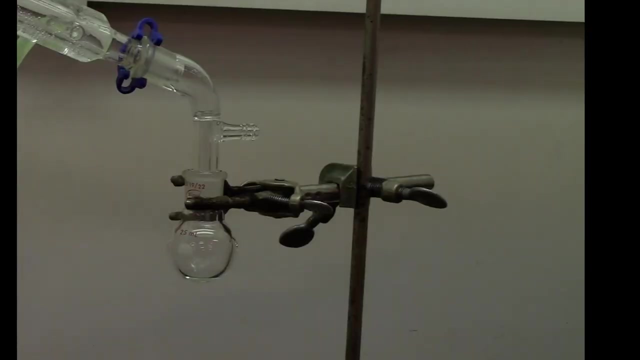 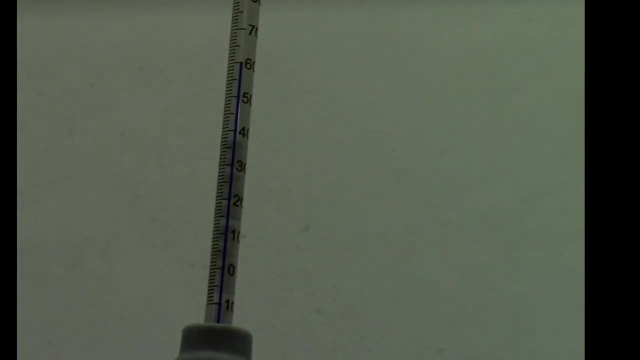 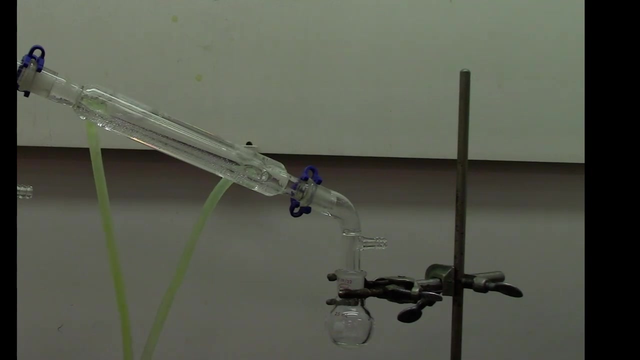 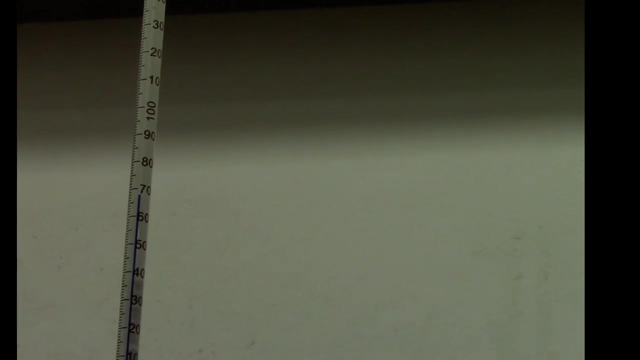 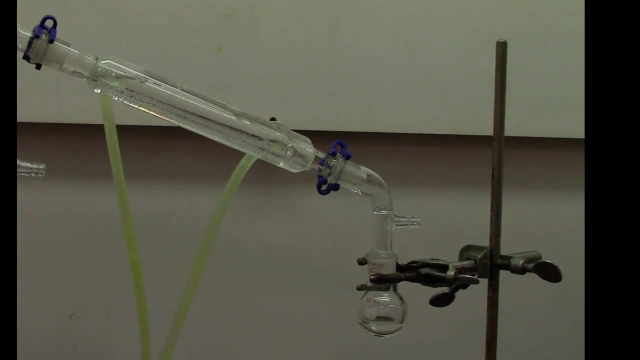 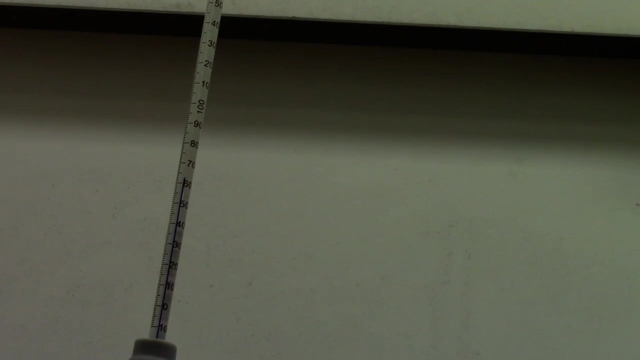 you, you, you. right now, the temperature is around 60 degrees celsius. now the temperature is around 70 degrees celsius. keep an eye on the temperature while it's still distilled. right now, the temperature looks around 62 degrees celsius, which tells most of the more volatile component, which is ethanol, has been distilled. 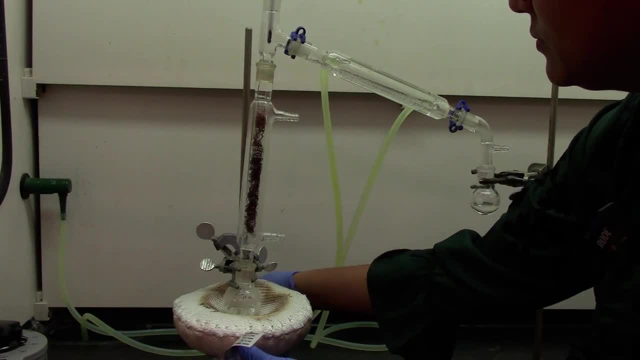 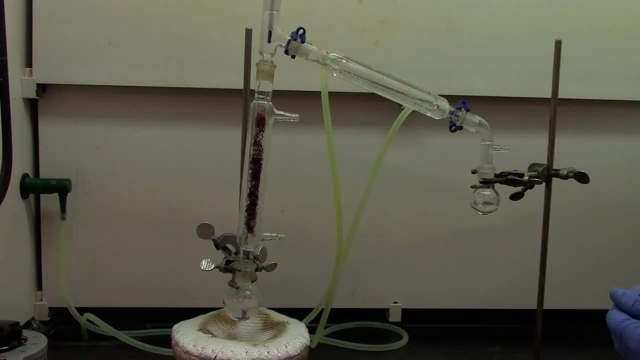 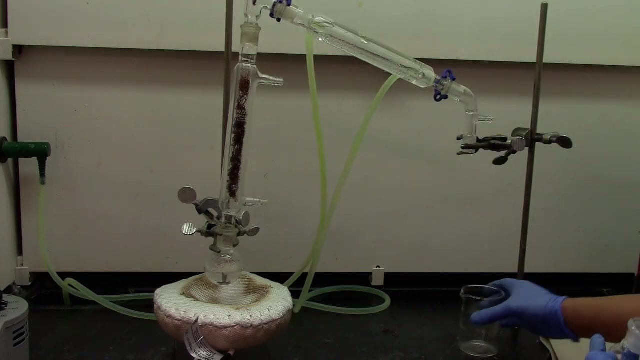 so it's a good time to turn off the heating and lower the mantle. we will go ahead and unclamp the collection flask. let the setup cool off for a few minutes before we start distilling. let the setup cool off for a few minutes before we start distilling. 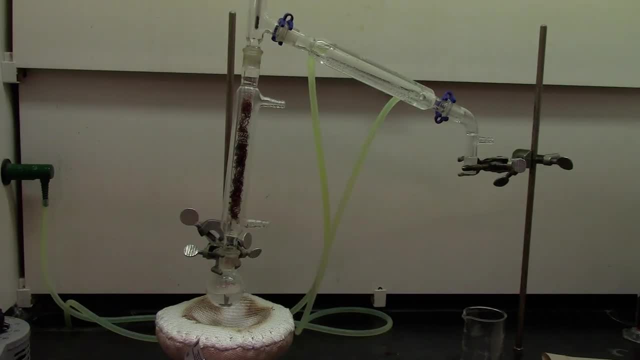 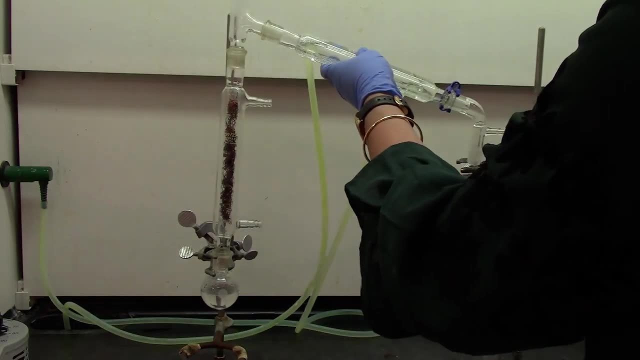 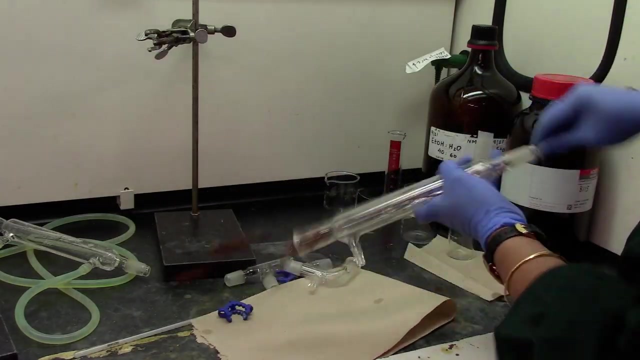 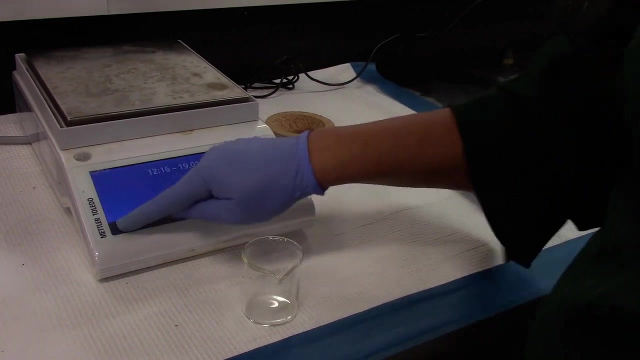 i am dismantling the setup. i am dismantling the setup. i am dismantling the setup. the copper turnings can be pushed from the distillation column and let it dry before it can be reused. we will go ahead and get the density of the distillate. 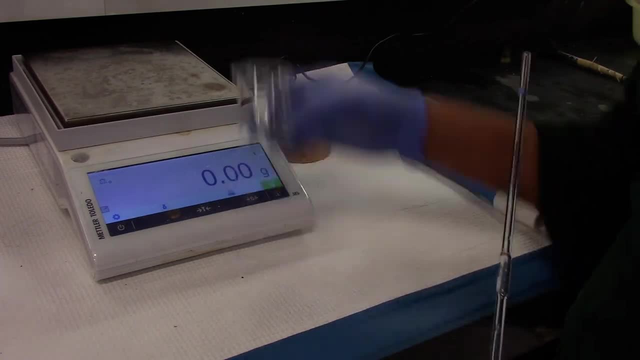 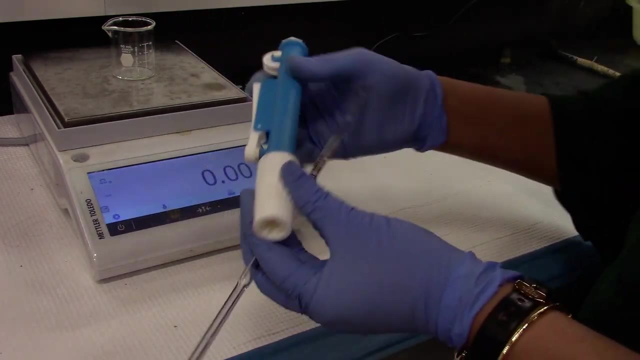 that we collected. that we collected in the 25 ml round bottom flask. So I'm using a small beaker, empty and dry. I'll tear the mass and use a one milliliter pipette with the auto pipetter and measure exactly one ml and get the. 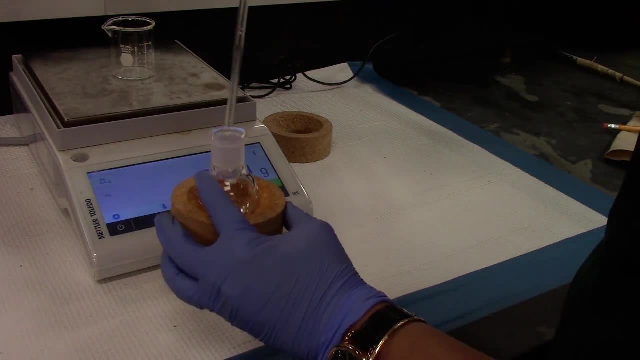 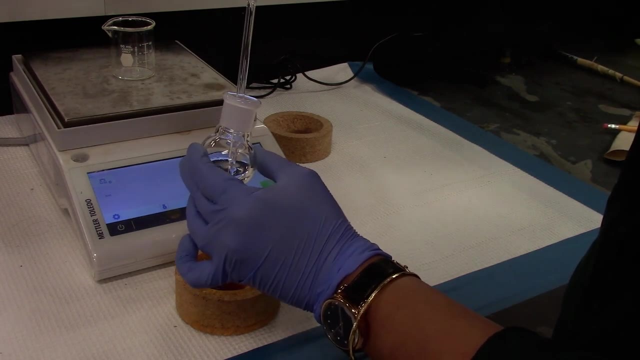 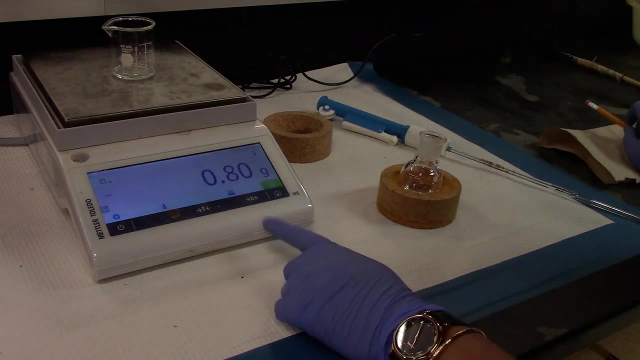 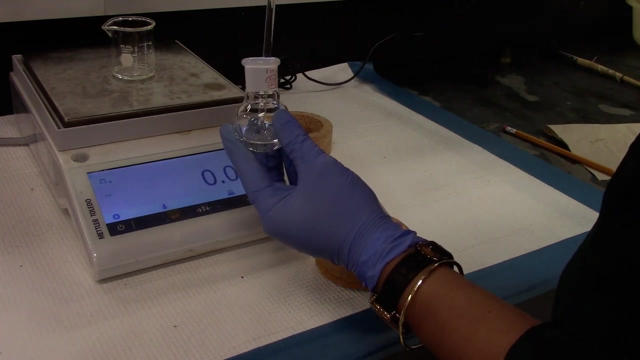 mass. So when you're measuring the density, it's grams per milliliter. That is what we are trying to achieve, measuring the grams for one milliliter solution. Go ahead and record the mass. We will tear the mass again and then add another one milliliter and 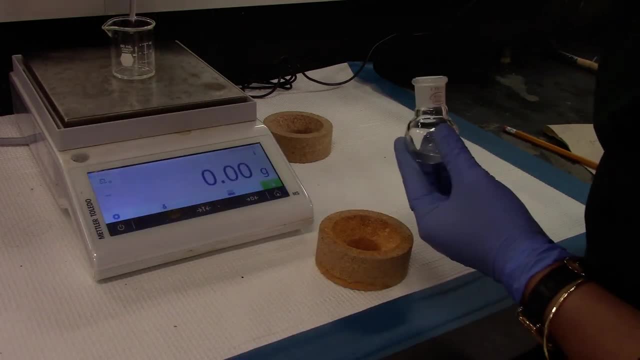 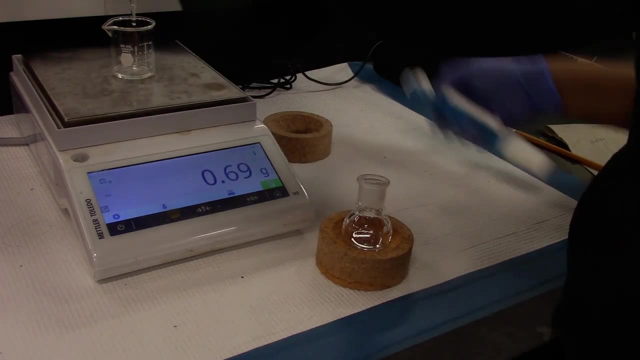 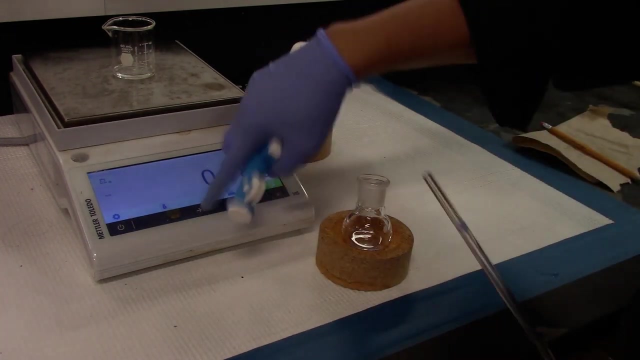 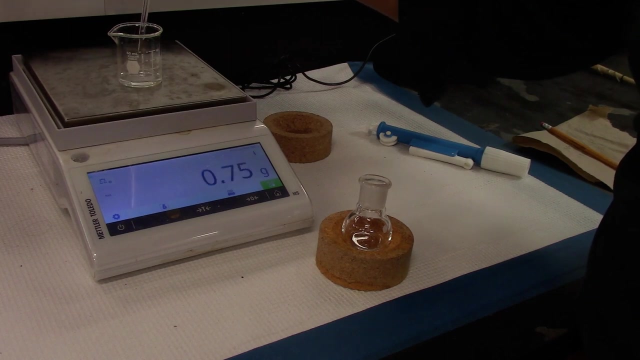 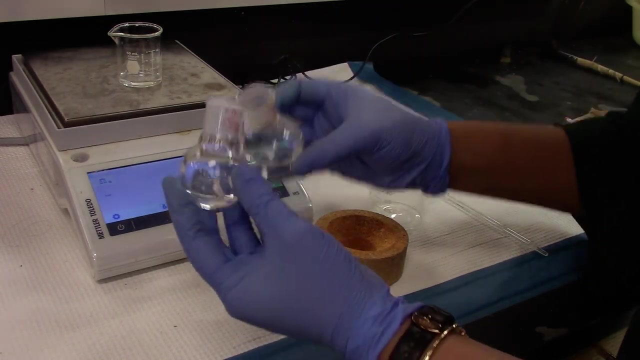 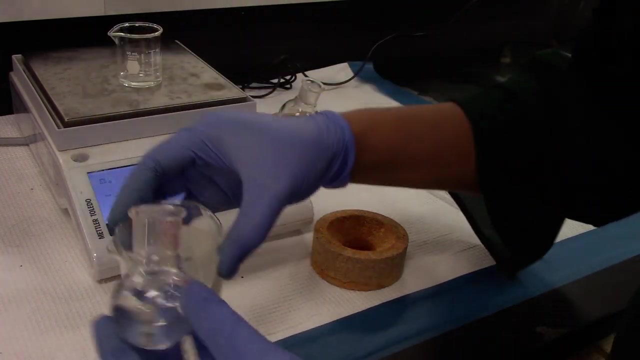 record the mass. We are doing three trials for measuring the grams for a milliliter solution: Tear the balance and measure the third trial At the end of the measurement. both the solutions can be combined and you can transfer it back to the beaker you collected it from, Since it's a mixture. 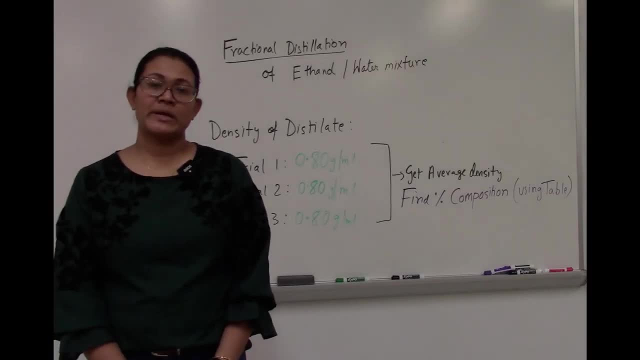 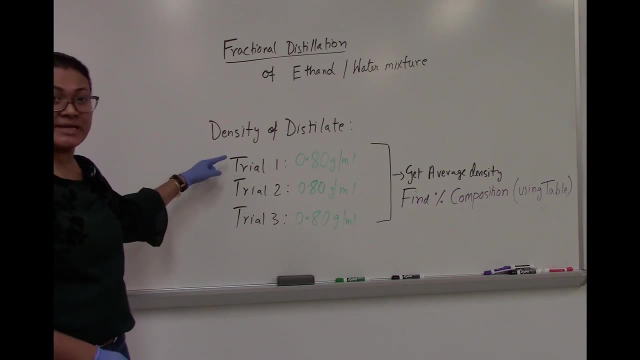 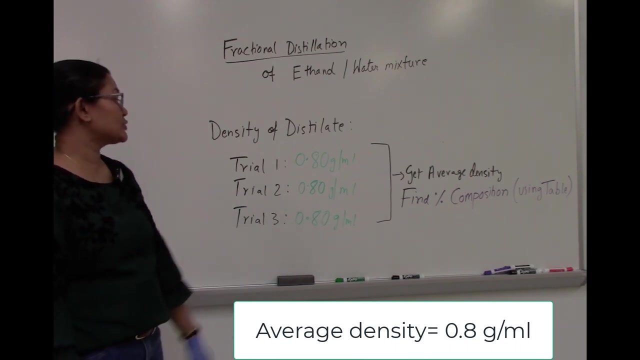 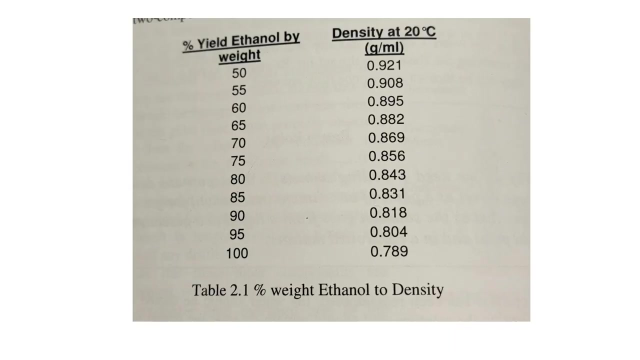 it can be reused. At the end of the fractional distillation we were able to separate the mixture of ethanol water and here are the results. And the results are politique technique paper. These are the three trials for the densities that we measured and the average density obtained was .8 g. whatever we use for the